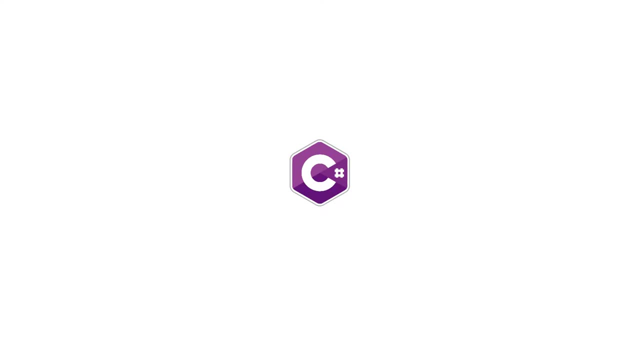 is in the description. We covered everything you need to know to be on the same page with me in this episode. It's very important to watch the first episode before you watch this one. Have you seen it? No, Then go watch it. Otherwise, thank you for being here. 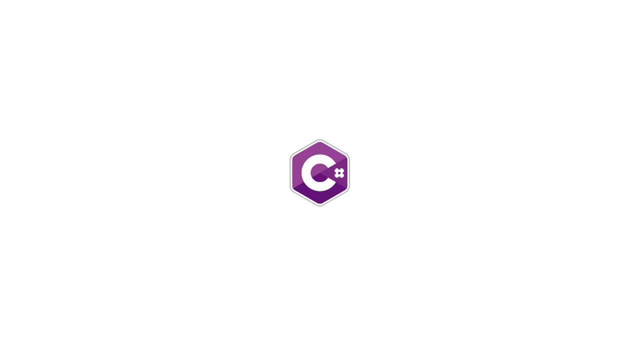 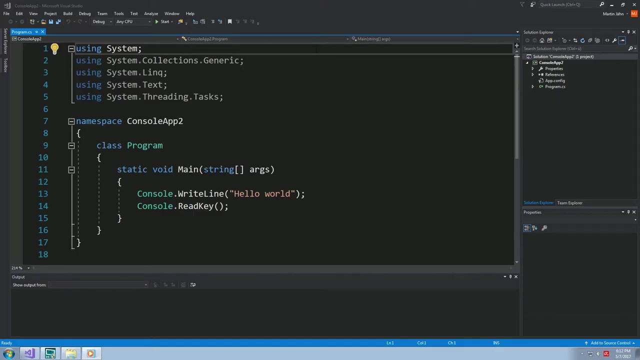 You are welcome. You are awesome. I appreciate it a lot. Thank you, Should we start, I guess? so right Here we have our code from the last episode. In this episode we will change a ton. You will see what I mean as we reach the end of the episode. 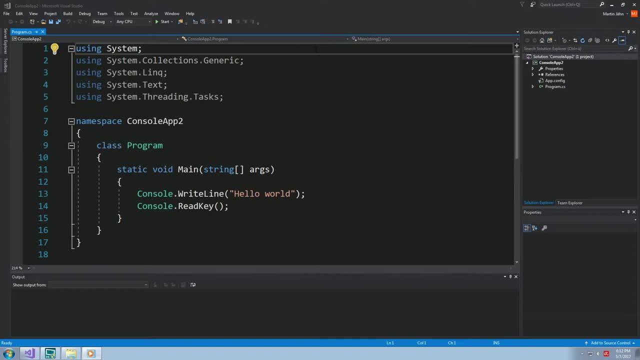 We are not only covering basic syntax here. no, We are also going to implement an example which also covers knowledge you learned in the last episode. Our goal for this video is to show you how to use basic syntax in C-sharp. For this episode is to create a rectangle class. This rectangle class will have different. 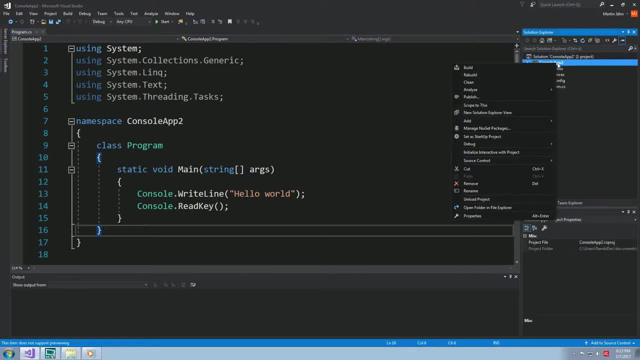 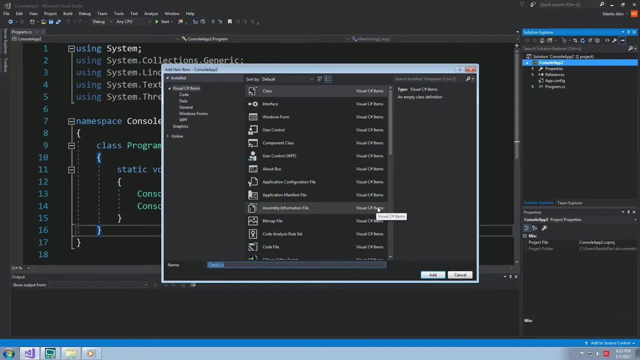 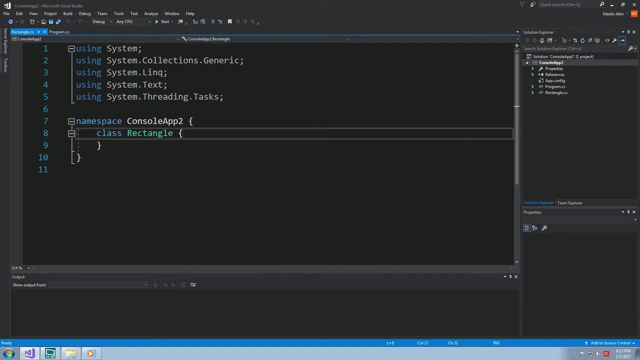 properties and two methods. One will display the properties and the other one will calculate the area of the defined rectangle. Be sure to be ready now, because this stuff is going to blow your mind if you never programmed anything. But please don't be nervous, Everything is going to be fine. Let's first declare some. 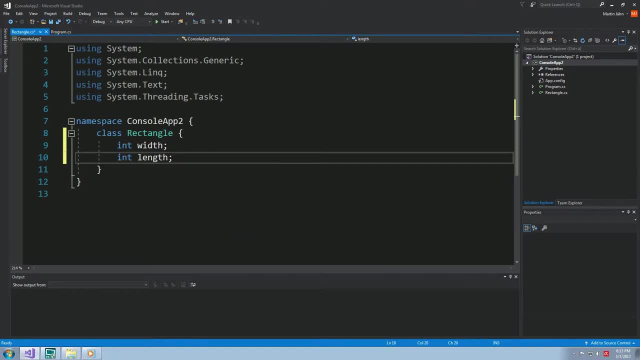 variables, An integer width and an integer length. What are these things? Sit back and listen. First things first, Let me tell you something about access modifiers. Access modifiers are in front of each variable, method and class, Virtually everywhere. There are four access. 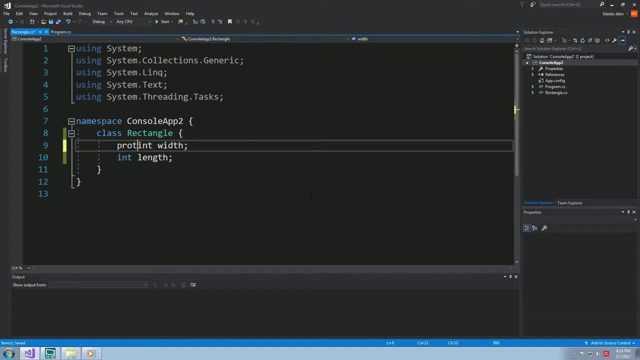 modifiers in total: Public, protected, internal and private. As the name access modifiers already tells us, they are modifying the access to certain things Like variables and methods. We are going to go step by step through some code in this episode and I will explain to. 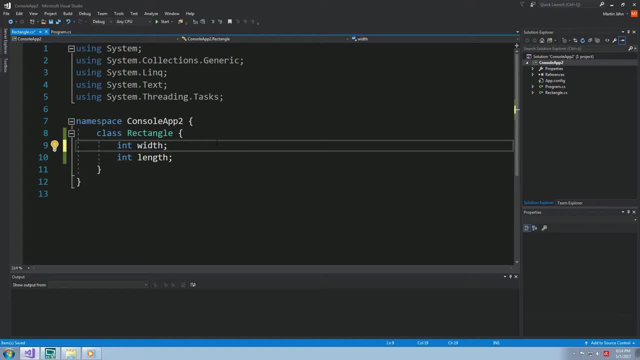 you when to use which modifier. Just one little but really important note at this point: Members without access modifiers are private. You are not allowed to use access modifiers for any of these purposes. If you could, you would ask me right now: Hey, what are you talking about? What are 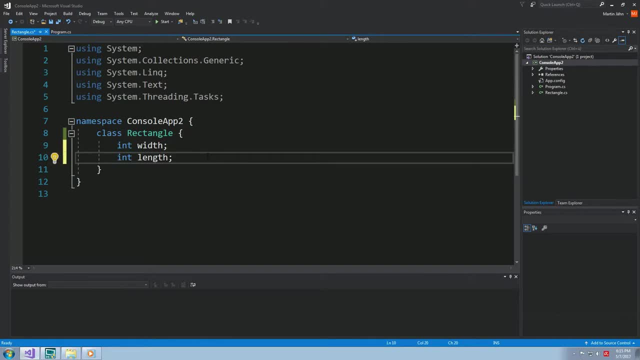 members, But it wouldn't be me if I hadn't already an answer to that. Members are basically variables and methods in a class. You might be familiar with the term variable because you attended some math classes. right, And actually it's not so far from it, To be honest. 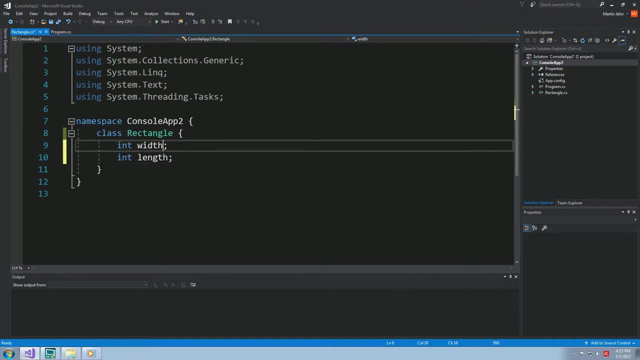 it's pretty much the same thing. Members are just different variables and they are all used to math and programming as well. So we have a major difference between math and programming variables. I'm sure you all know what I'm talking about For everyone else. don't be ashamed, it's ok, I'll explain it anyway. 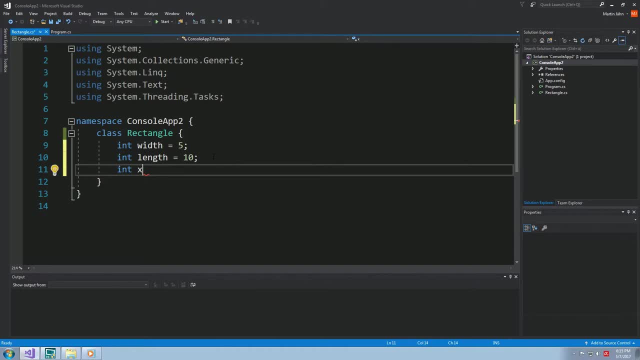 You're probably used to coordinate variables like X, Y and Z. However, in programming we can use verbs to describe our variables, not only single letters. You probably already knew that anyway. But hey, I'm covering everything. Enough math references, I will focus on programming. 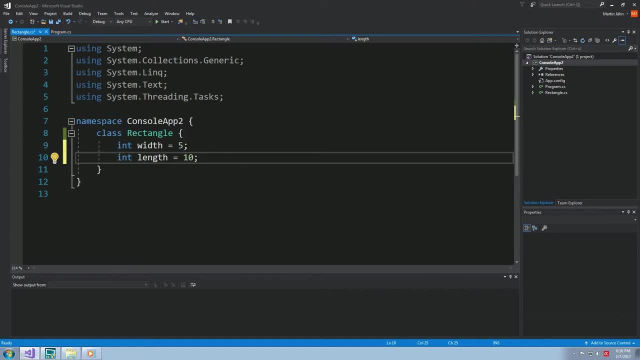 now, I promise. What else do we need to declare a variable? We need a data type. Let's have a look at data types, shall we? With data types, we can specify what form of values can be stored in a variable. They are also seen in the declaration of functions, which then? 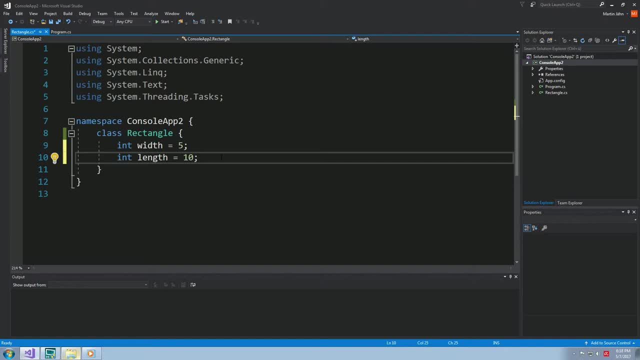 specifies the return type of this function. Instead of hitting you in the face with a table of data types, I list some of the most common ones: Strings are text, integers are numbers without decimal places, floats are numbers with decimal places and bools are: 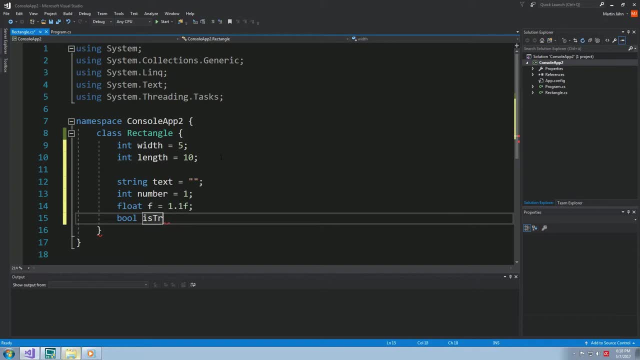 either true or false. Remember these data types and you can almost do anything you want. Let's get into some boundaries of these number data types. Integers go from minus 2 billion 147 million 483 thousand 648 to 2 billion 147 million. 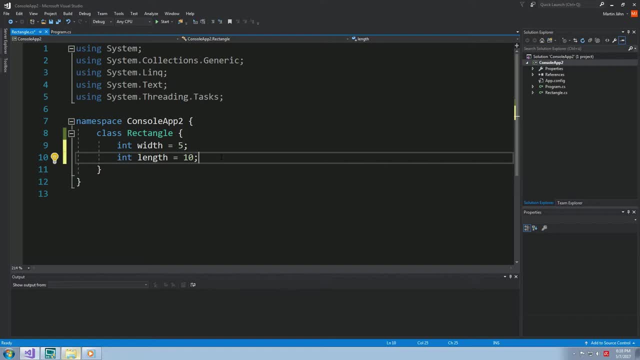 483 thousand 648.. Floats from minus 3.402823 times 10 to the power of 38, to 3.402823 times 10 to the power of 38.. Okay, let's move on. Wow, these are quite some numbers. 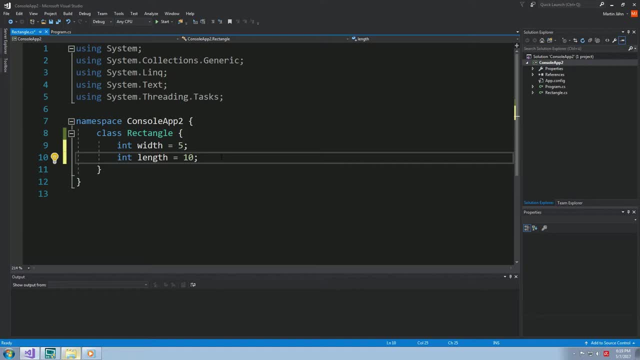 If you are interested in other data types in C-sharp, check out the link in the description. Now we need that method I mentioned earlier, The method which displays the values stored in the variables. This is how we declare this method Public void display. 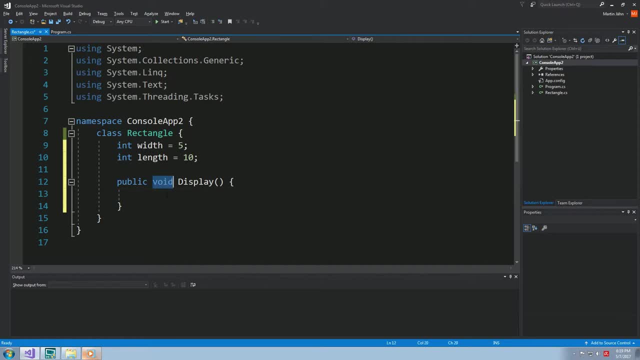 Void means there is no return type. The method doesn't return a value, it just processes the code which is in its body. We will declare a method with a return type later in this episode. Why do you have to use public, you ask. 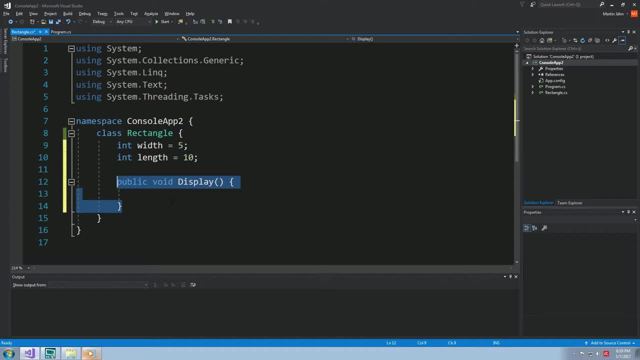 We have to use public to be able to call the method from another class, which we will do later in the video. As you know, consoleWriteLine writes a message to the console, So let's use this to display the property ConsoleWriteLine text width plus the variable width. 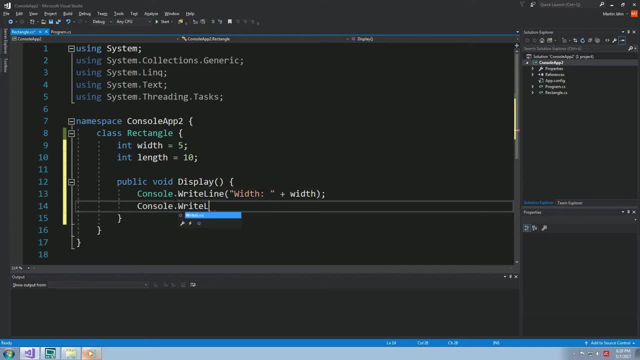 And consoleWriteLine text length plus the variable length. No, I am not trying to add the length variable to the text length. In this case, the plus just concatenates the text and the variable Or the value of the variable. We want to implement the second method. 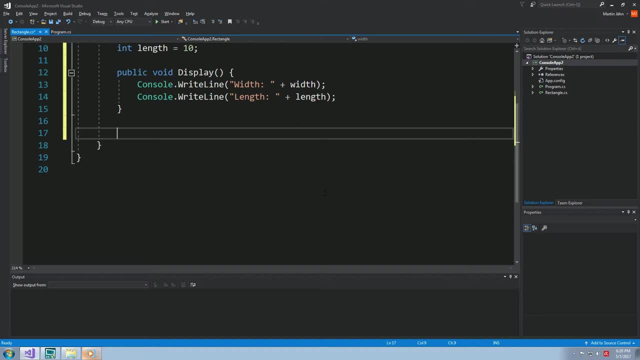 The area calculation. I don't think I have to explain how to calculate the area of a rectangle right, Because we don't have a variable to store the area. No, no, Don't create an area variable now, Just don't. 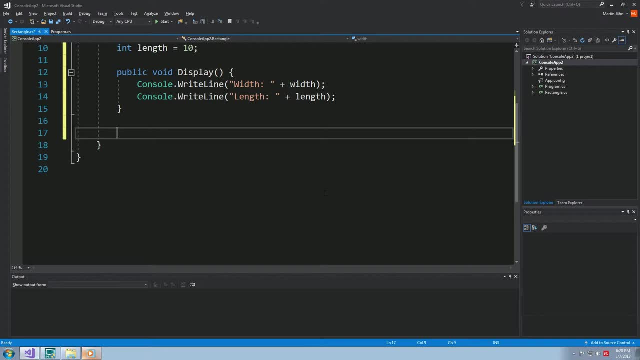 This destroys the purpose of this tutorial series. if you do everything on your own, Ok, Everything is fine. They are listening to me. They do what I explain. Ok, Because we don't have a variable to store the area, we declare this method with a return. 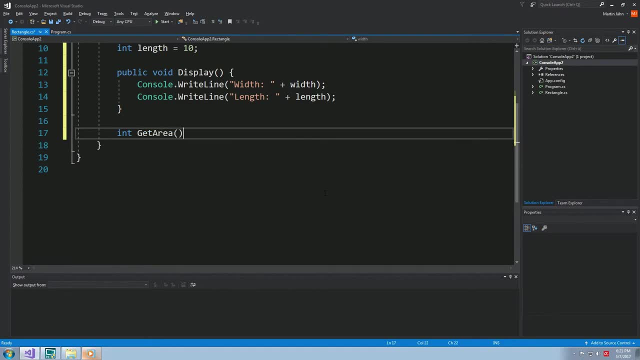 type. This method will return an integer int: getArea. In order to return something, we need the return keyword. Return width times length. We need the return keyword. Return width times length. We now need to go back to the display method and add a new line of code. 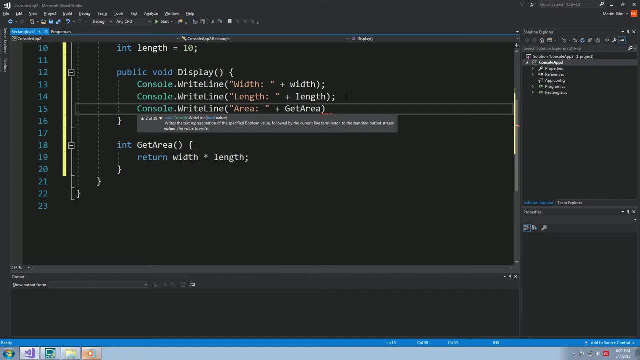 ConsoleWriteLineTextArea plus the method getArea. Here's something else I just want to throw out. now There's another syntax for the whole writing thing we are doing three times in this method: ConsoleWriteLineWidth, curly bracket zero And the variable width as a parameter. 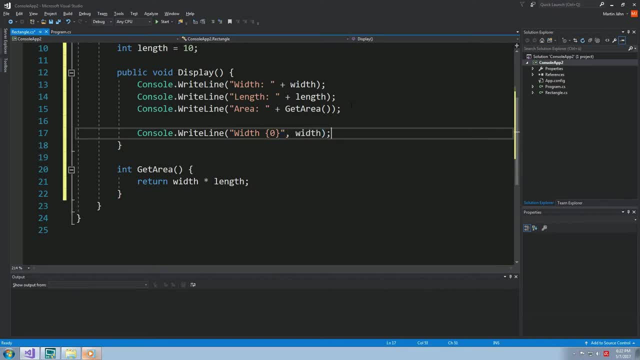 This is doing exactly the same thing, except the message is concatenated in another way. It takes the value from the width variable and puts it in the place of curly bracket zero. So with this we could do something like that: ConsoleWriteLineWidth- curly bracket zero. 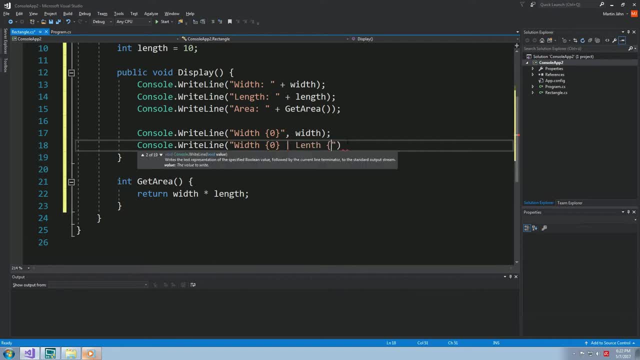 Vertical line Length, curly bracket one. Let's do that. Ok, Let's get the text in. Let's say we want length and width as the parameters. In the other syntax it would look like this: ConsoleWriteLineTextWidth plus the variable width plus text. vertical line length plus. 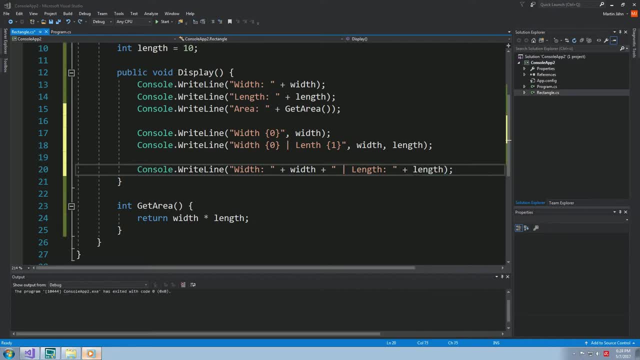 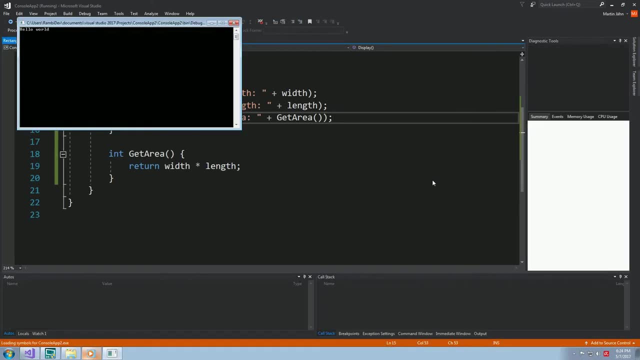 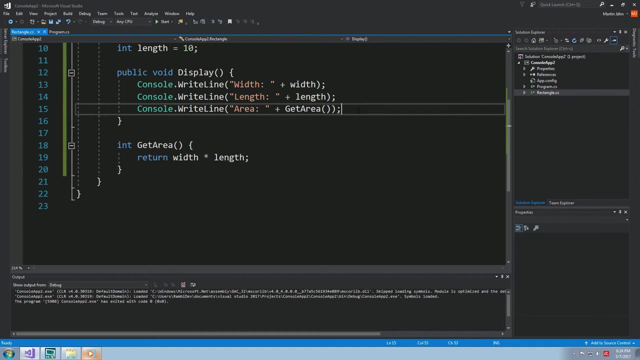 the variable length. Ok, Great, All done. Right, Let's test, Let's see how it's going. Oh, no, what? this is not the output we expected, is it of course not? why, as you learned in the last episode, the main method is the entry point for C sharp programs. so 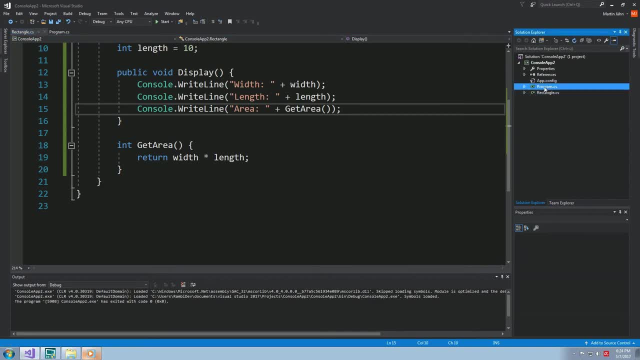 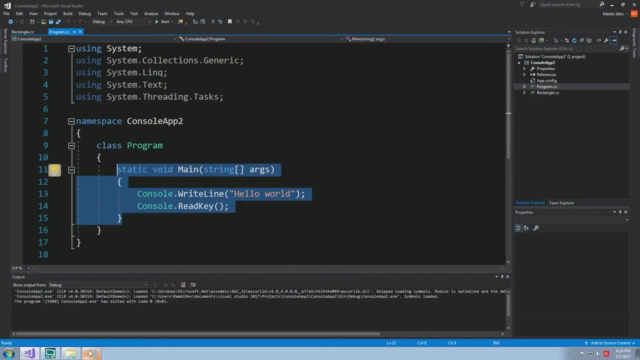 let's have a look there and see what we can find. Oh, still the code from the last episode. how miraculous. no, actually not, I'm, I'm sorry. and this brings us to instantiation of classes. does that sound complicated to you? it doesn't. wow, that's good. I can already feel your programming skills. what is instantiation, seriously? 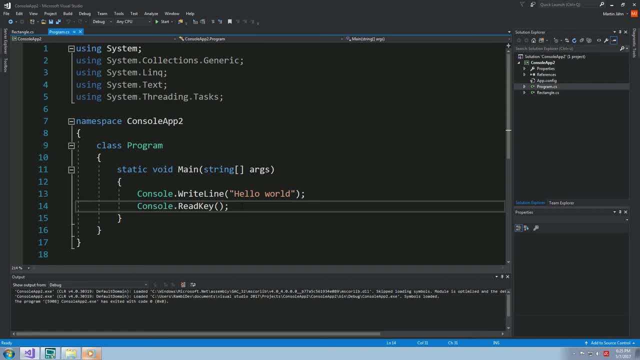 now I will kill the script writer for using that word so often. instantiation of classes is a very common word in the world of programming. instantiation of classes is a very common word in the world of programming. instantiation everywhere. I hate it. what I should continue the episode? oh, yeah, you.